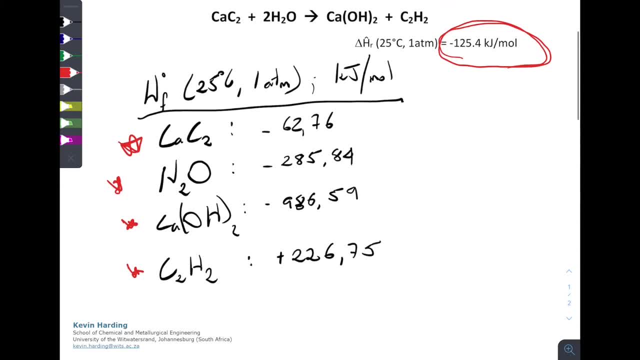 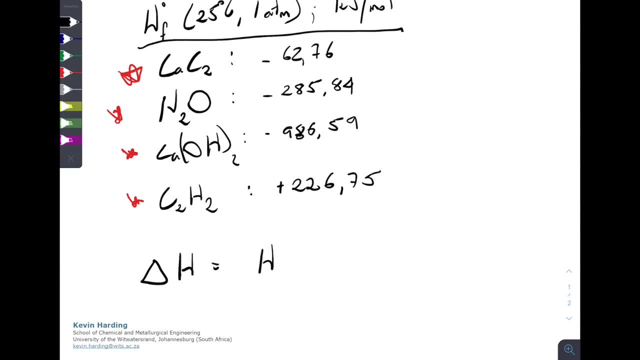 worked out the difference in enthalpy just from these numbers. I would do the following: I would want to look at the delta H, so that's the change across it, and would start out by the enthalpy or the change in enthalpy of the products. 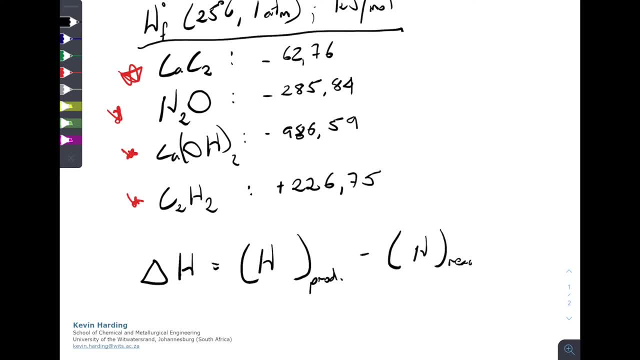 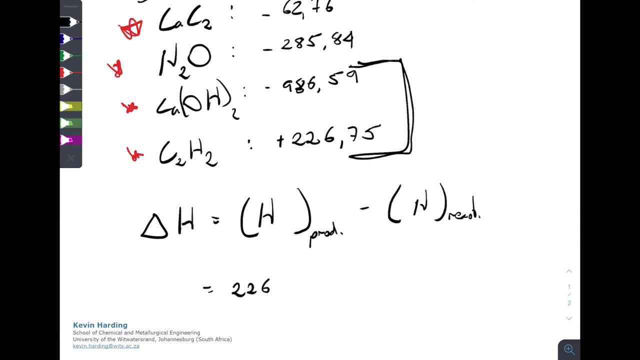 Minus the enthalpy of the reactants. In this instance the products are these two on the bottom here, so that's simply going to be 226.75 plus the negative value. so let's rather write that as minus 986.59, so that's the enthalpy of the products. We are then going. 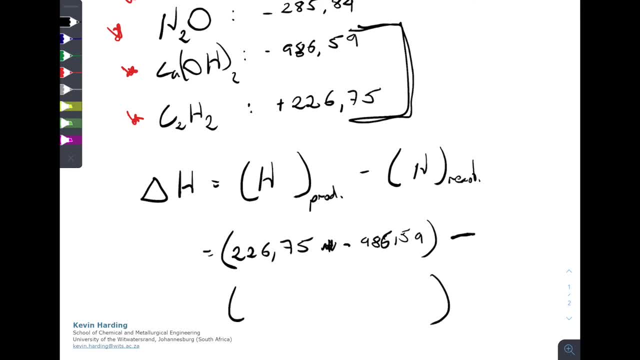 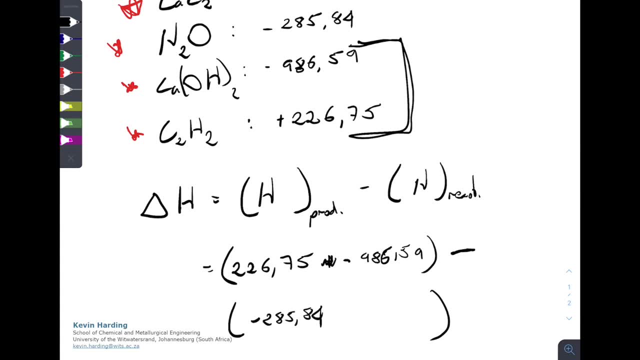 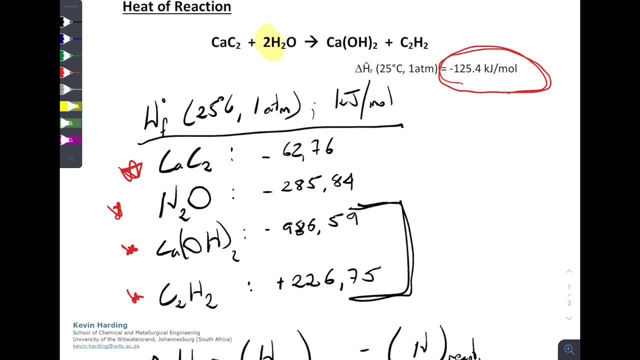 to subtract the reactants, and that is the water, which is minus 285.84, but I need to remember that up at the top here we had that, the water. there were two waters in this reaction, so I need to multiply this value by 2.. 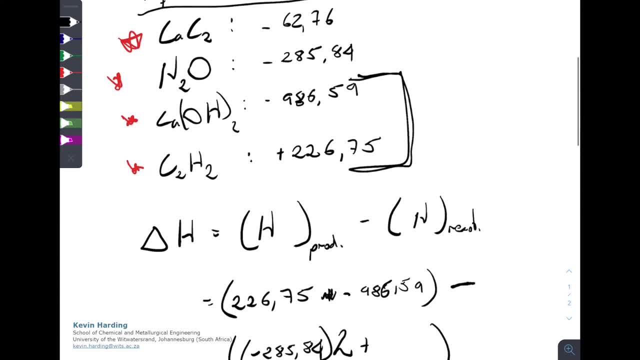 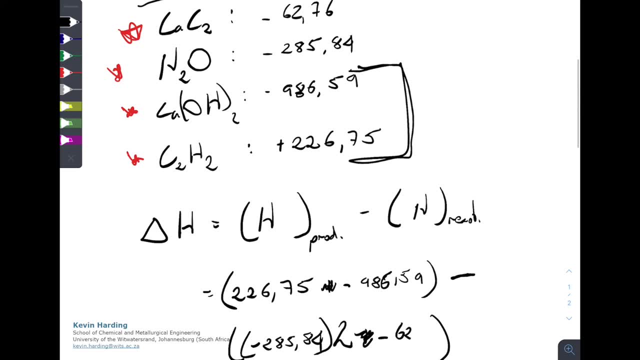 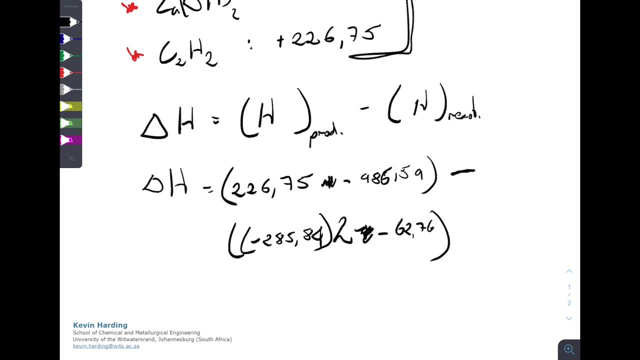 And then I need to add to that the calcium carbide value of minus 6276, so again, let's just put that as minus 62.76.. change in enthalpy across that system. and remember this was all at 25 degrees Celsius for the. 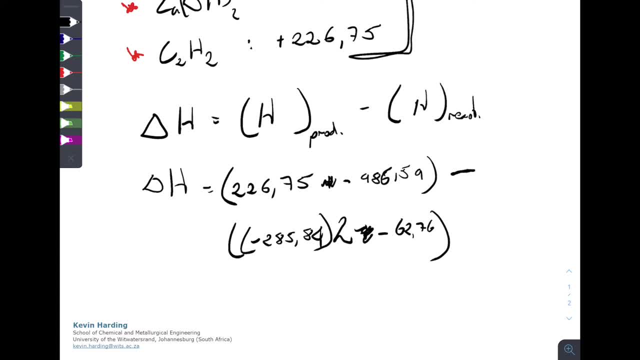 products and the reactants, and it was 100% conversion. If I do this on a piece of paper next to us, the final answer on this is minus 125.4 kilojoules per mole and if you look at that, that value there- 125.4 kilojoules per mole- is exactly the same value as the 125.4 kilojoules. 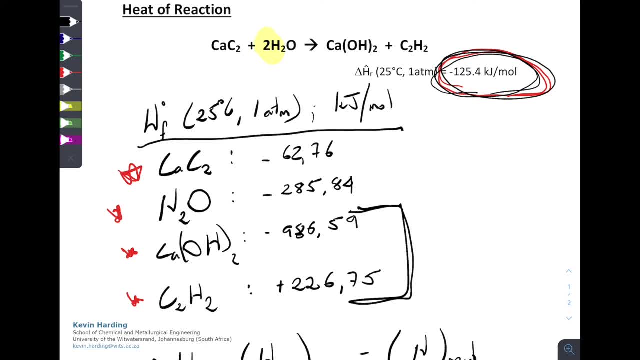 per mole, as we were given in a table before. The one thing that I cannot stress enough is that the value 125.4 had to be for a 100% conversion. The inlet and the outlet, so inlet plus the outlet, temperatures were all at 25 degrees Celsius. There was no excess, there was no, nothing else that was. 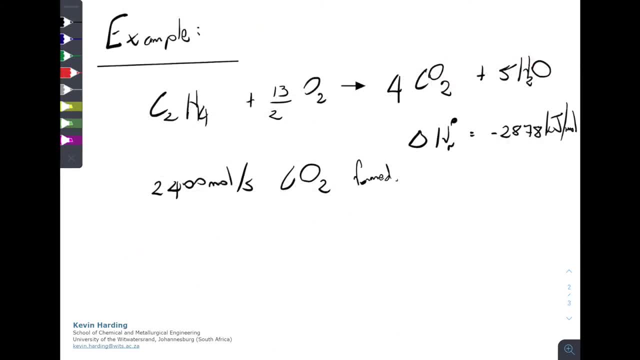 coming into that system. If we look at a quick example on how we might use this, here is the example of C2H4 reacting with oxygen to form carbon dioxide and water. In this equation, we are given that the delta H of reaction is equal to minus 2878 kilojoules per mole, and we are asked: 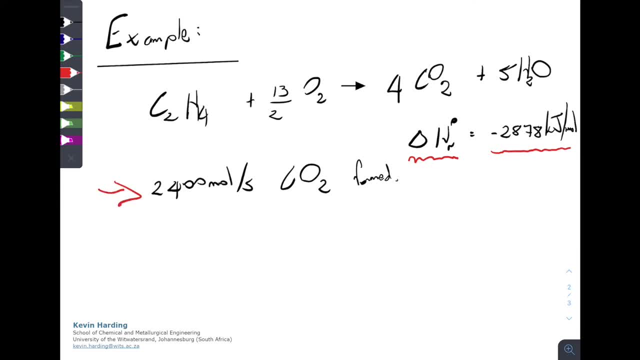 if there is 2400 moles of second per second of carbon dioxide forming, what is the delta H for this reaction? So the first thing to notice is that on this equation, the delta H of reaction is given as a per mole. So, because it's given per mole, what that means is it comes with this. 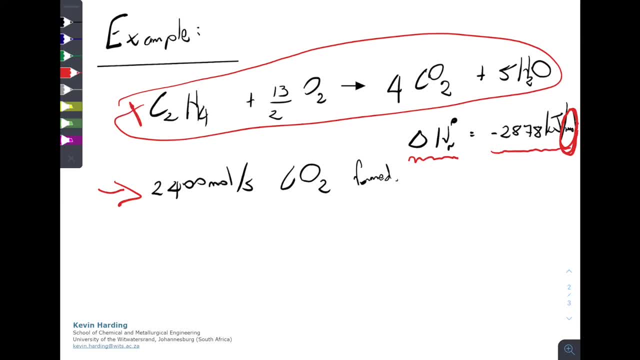 reaction. So it means that for one mole of C2H4, 13 on two O2s, four carbon oxides and five hydrogens, that's how many kilojoules are required for the heat of reaction. So in other words, what we need to look at is, for this, 2400 moles. that relates to the CO2.. So, because that relates to 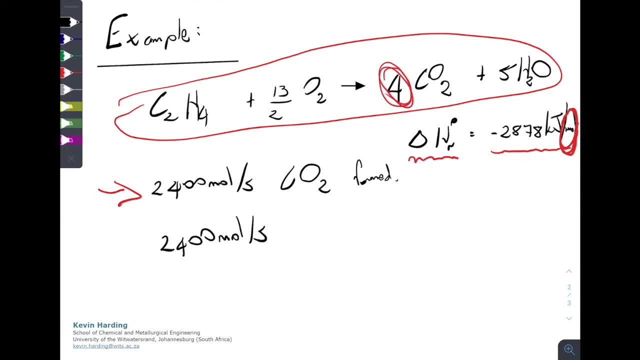 the CO2. the coefficient in front of it is four, so we need to divide that by four To give us the actual extent for this reaction. The delta H of that would then be equal to that 2400 divided by four, multiplied by minus 2878, which will equal minus 173- sorry, 1.73 times 10. 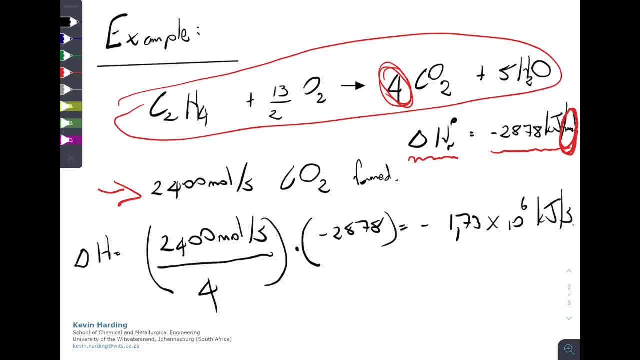 to the 6 kilojoules per mole. So that's the actual extent for this reaction. So the delta H of that 2400 is equal to that 2400 moles per second. If this question had said that the information here 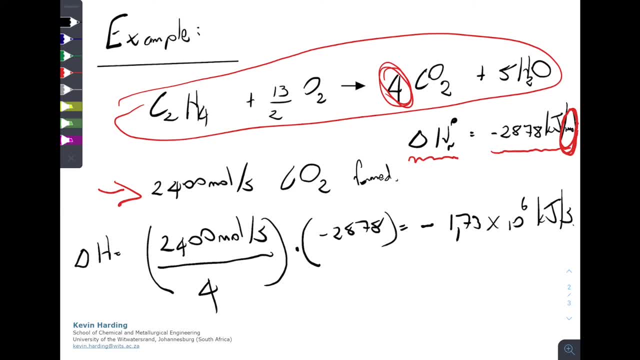 was the same, but the products or the reactants were coming out at a different temperature. we would have to approach this slightly differently. In that instance, we would not be able to use the delta H of reaction, and this would all have to change. So what we would then do is the same way. 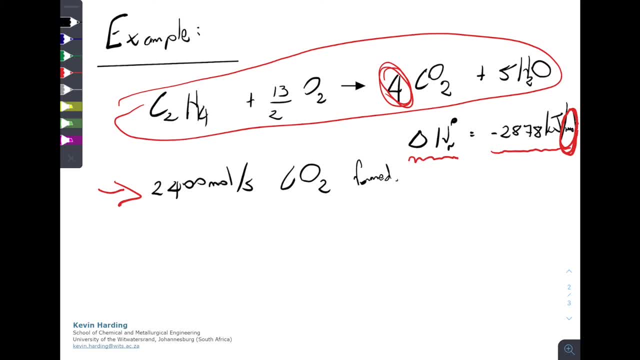 as we calculated or we checked the delta H previously, where the delta H would have to equal to the change in H of the products minus the change in the delta H of the reactants. In that instance we would have to look at the delta H of formation and if there is a change in the